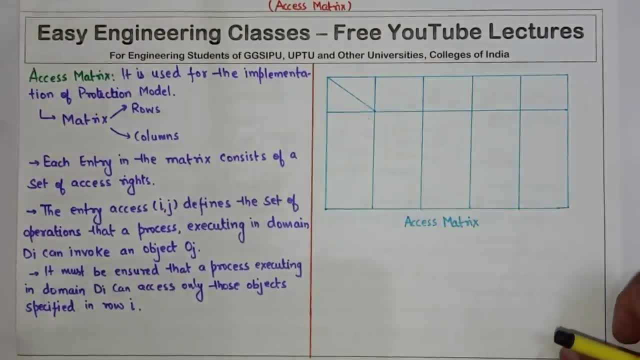 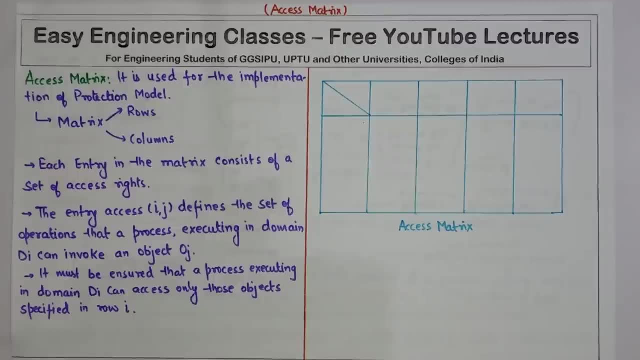 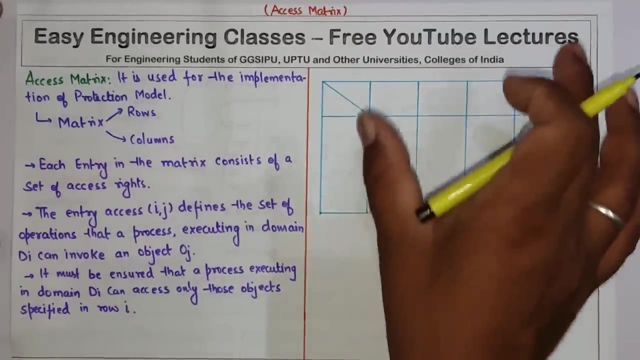 Hello everyone, today in this video we are going to see the access matrix which is used for the implementation of the protection model which we have studied in the previous lecture. So this is access matrix. We are going to see the entries, that, how it is filled and what are those entries and what is the meaning of those entries. 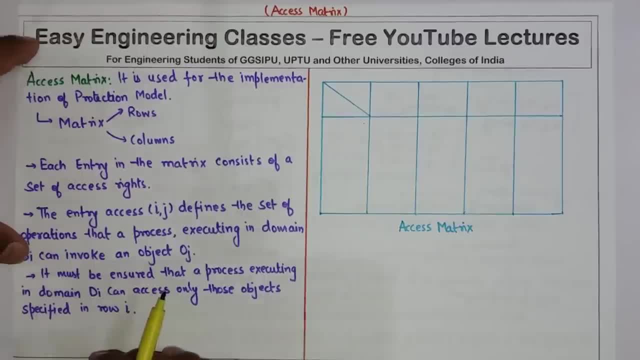 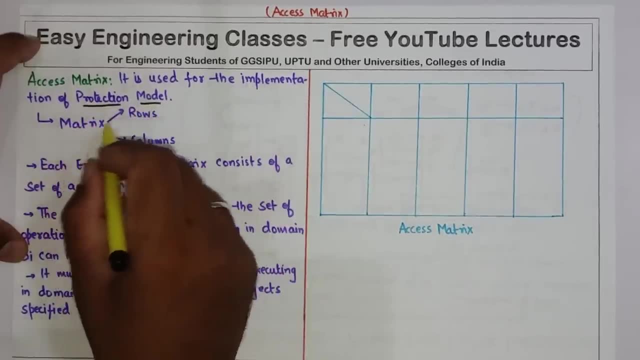 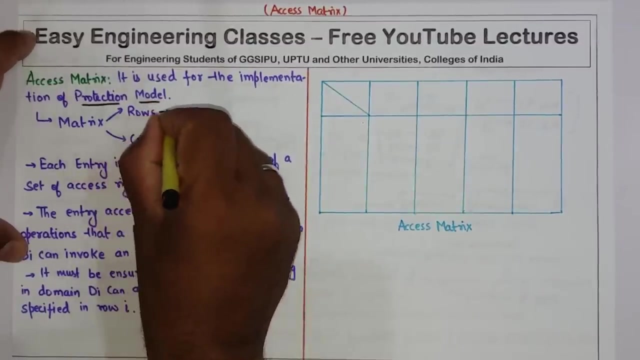 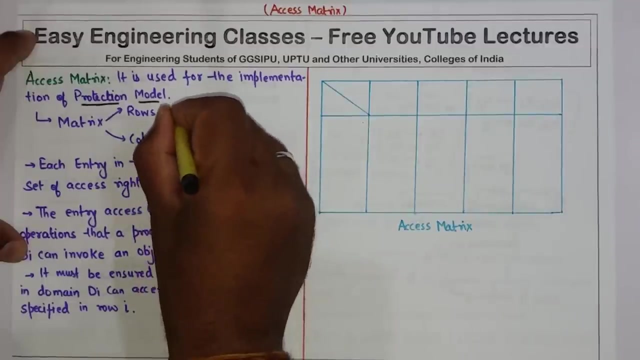 Now, first we see some of the theory aspect of the access matrix. So access matrix is used for the implementation of the protection model. In any matrix there are two different entries: One is rows and another is columns. So the row which we are going to define it like this: These are used to represent the domain. 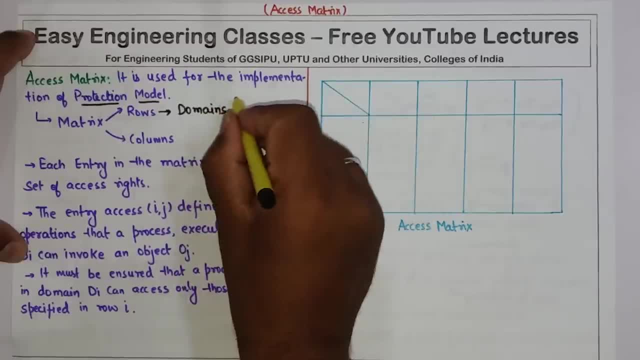 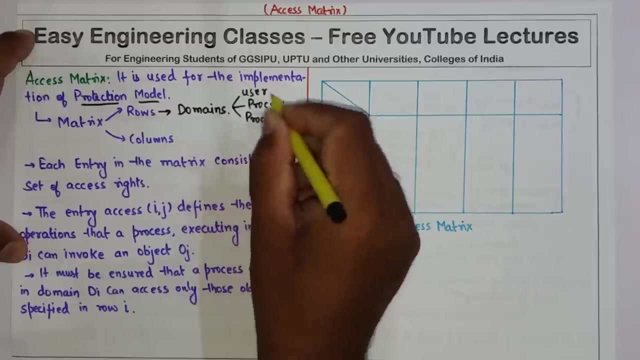 So these are used to represent the domain And we have seen in the previous video that there can be different kind of domains, like there can be a user domain, there can be a process domain and there can also be a procedure domain. So any of those three kinds of domains are represented with the help of rows in the matrix. 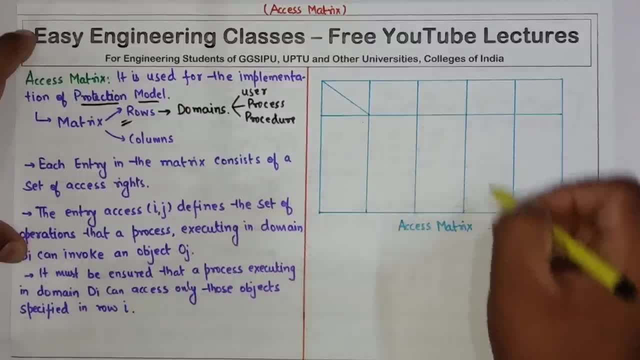 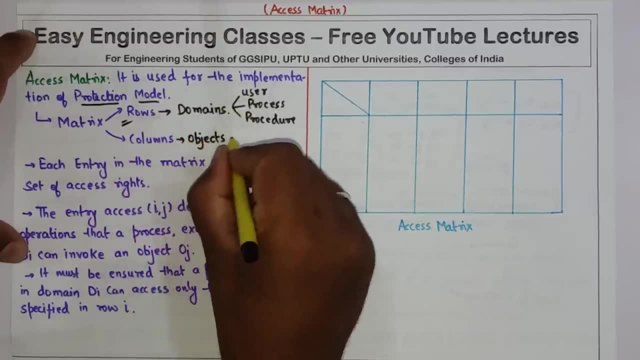 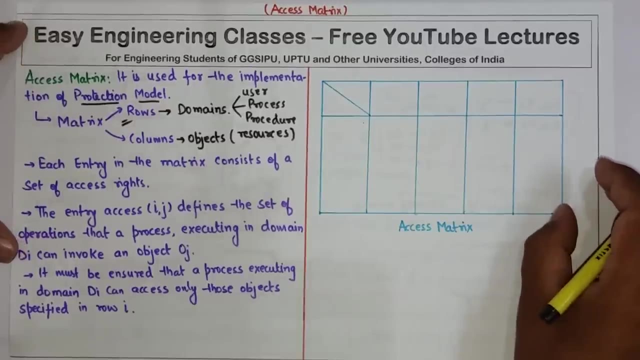 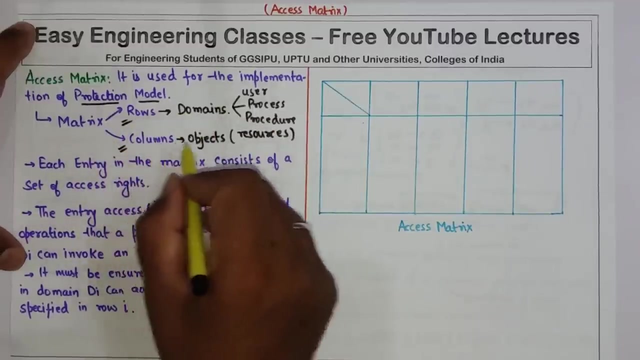 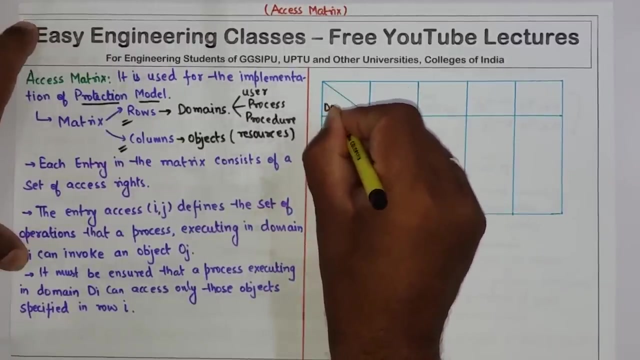 Then there are columns like this. So these columns are representing the objects And these objects are actually the resources that are present in any operating system. So clearly there are two different entries: One is rows representing domains, and another is columns representing objects. So now, if we fill this, So we are going to represent domain like this and objects like this. 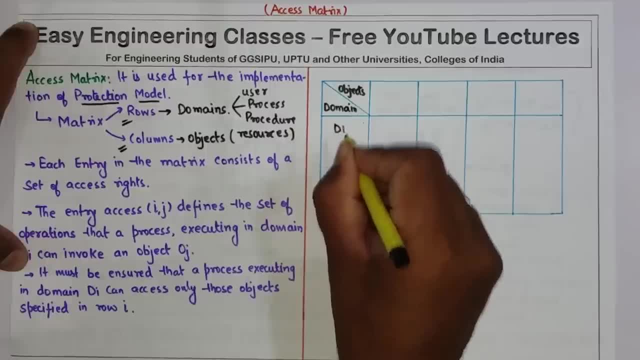 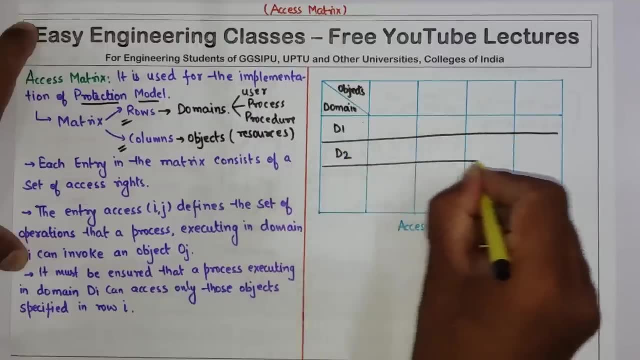 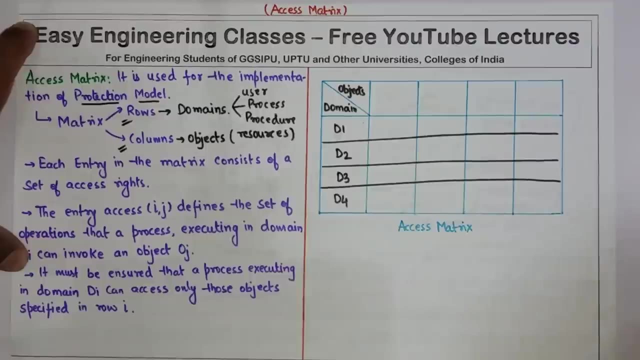 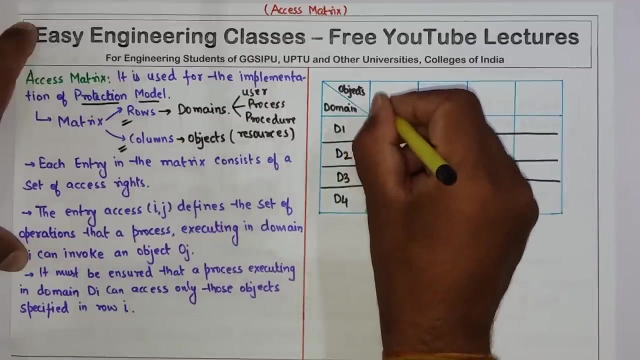 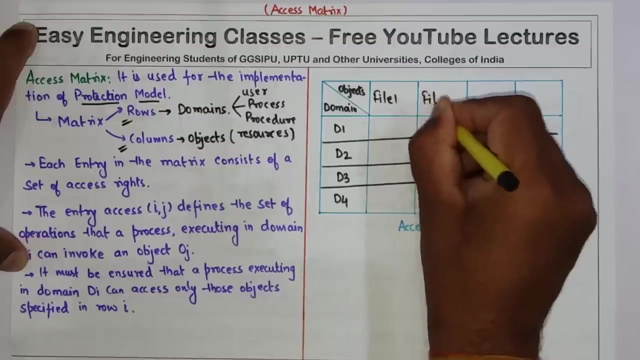 So suppose we have four domains: D1, D2, D3 and D4.. So these are the four domains that we have specified in the rows, And the objects are like, suppose, file 1.. Then we have this file 2, file 3, and one object can be a printer. 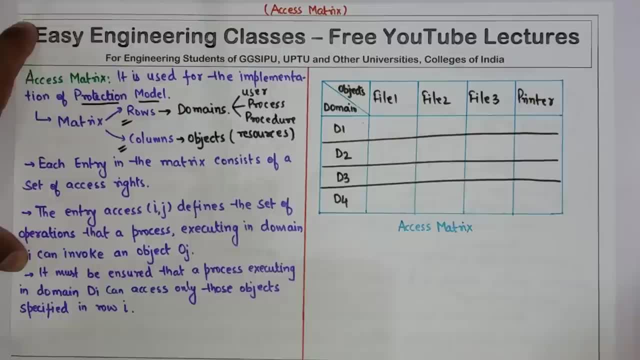 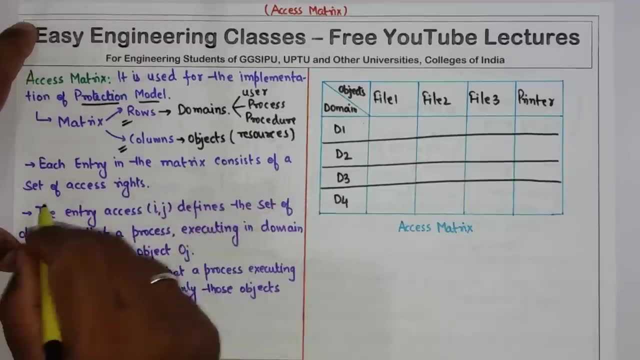 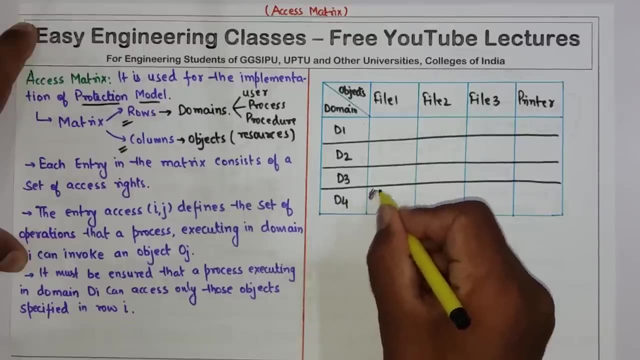 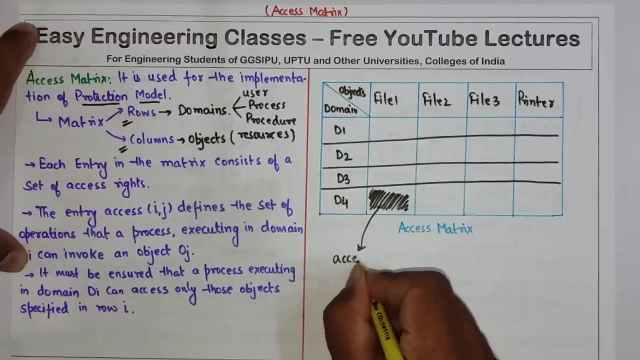 So these are the domains and these are the objects. Now, each entry in the matrix consists of the set of access right. So each entry in the matrix- So, for example, this entry, This entry- This entry will consist of what? Access right information. 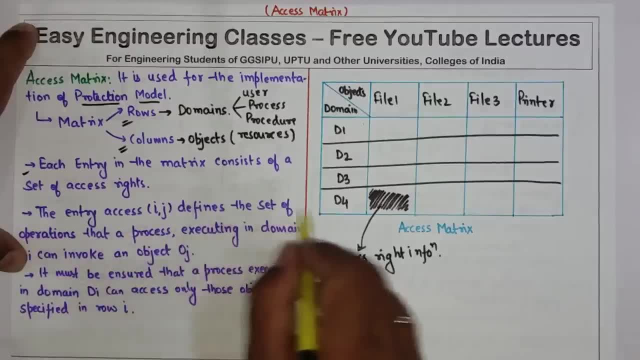 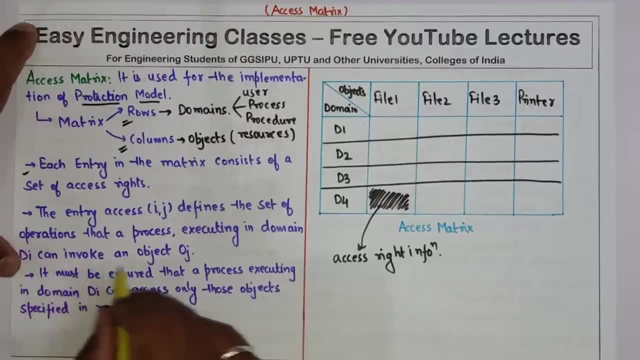 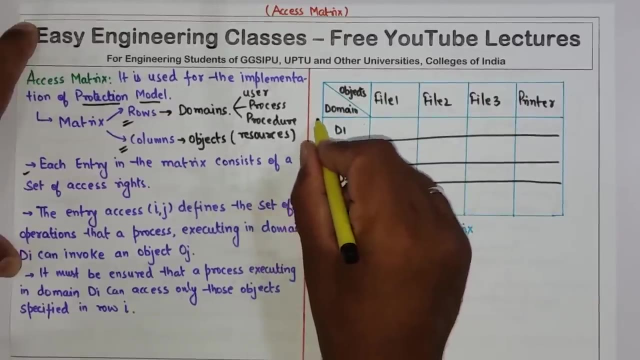 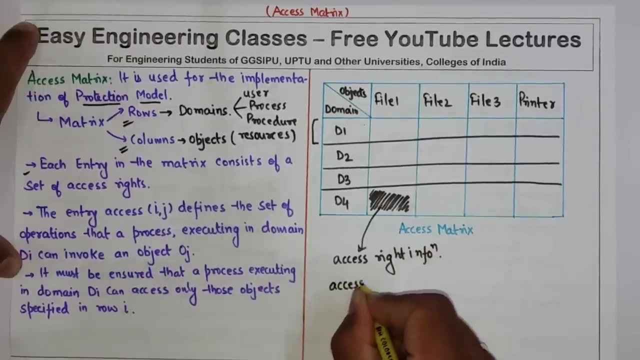 The entry access IJ defines the set of operations that a process executing in the domain DI can invoke an object OJ. So, for example, a process is executed In this domain D1,, so I is 1.. So if I am writing it like this: access 1, comma 1.. 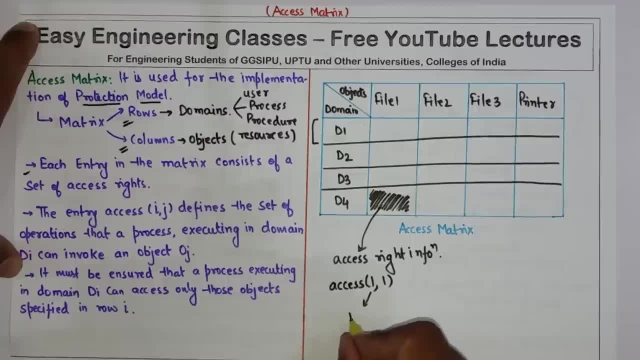 So what we are I am representing is: this is I, this is the domain 1 and this is object 1, because J is 1.. So I am representing like this: So it means that this- the process executing in this domain 1. Can access the resources in this object 1.. 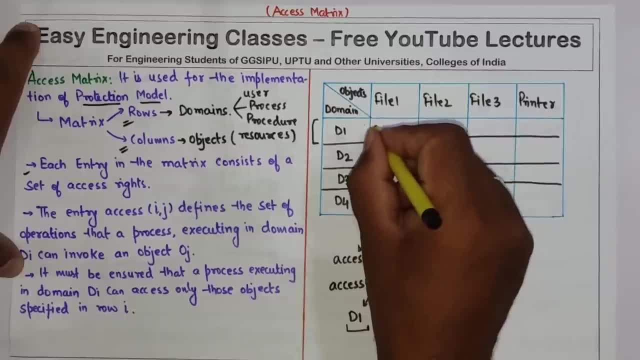 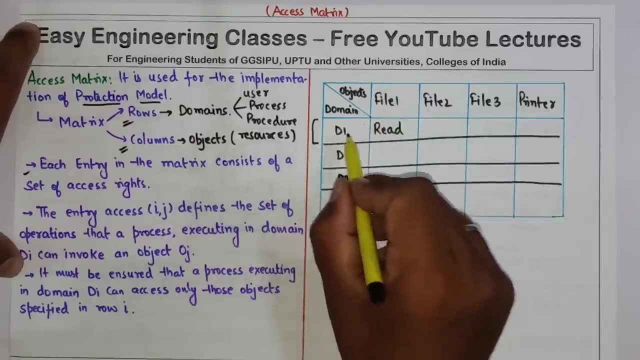 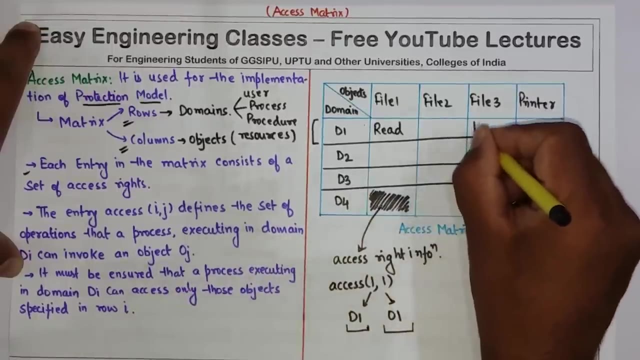 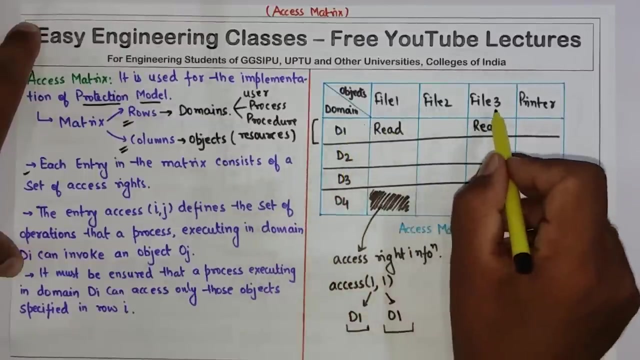 So, for example, if I have an entry like this: read, it means that a process executing in this domain can read file 1. Clear. Similarly, if I have an entry like this: read, it means process executing in this domain D1 can read file 3.. 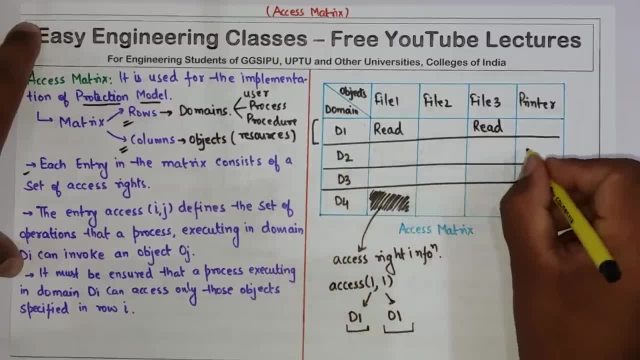 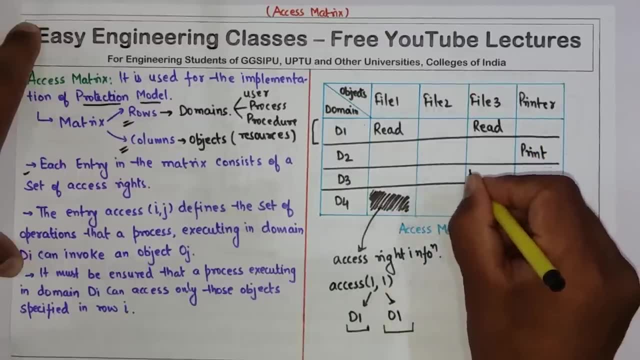 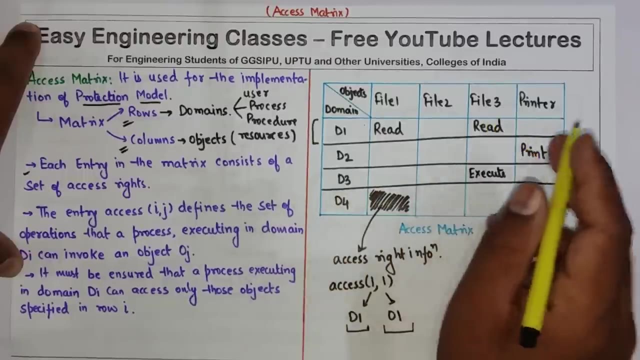 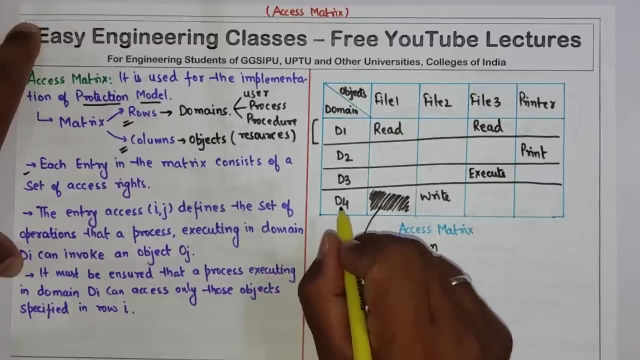 Similarly, if a process executing in domain 2 can give command of print. Similarly, if I give execute here, it means a process executing in domain 3 can execute file 3.. Similarly, if I have a write, here, it means a process executing in domain 4 can issue write operation on file 2.. 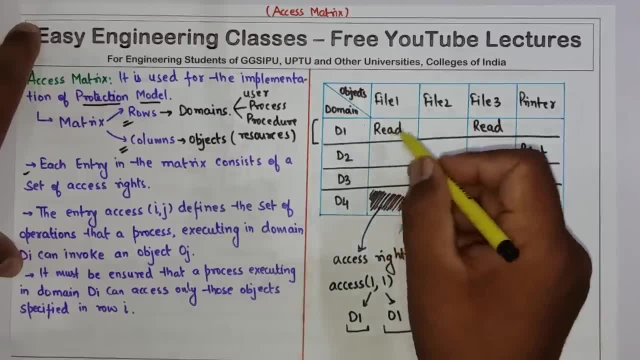 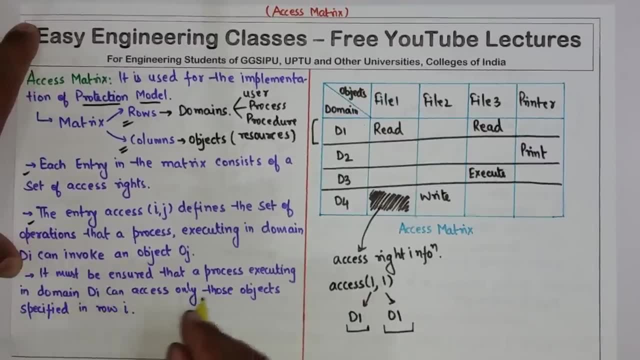 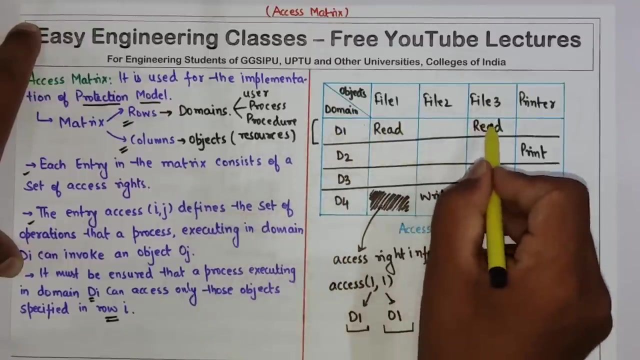 So in this way the Access matrix work and each entry is representing the access write information. Now it must be ensured that a process executing in the domain D I can access only those objects specified in row I. So what it means is, if I have an entry like this, it means D1 can only read file 1 and file 3..